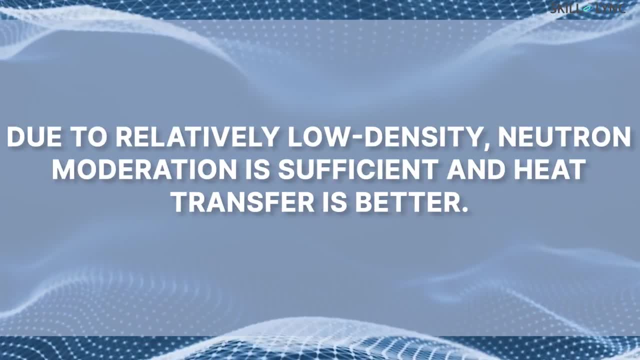 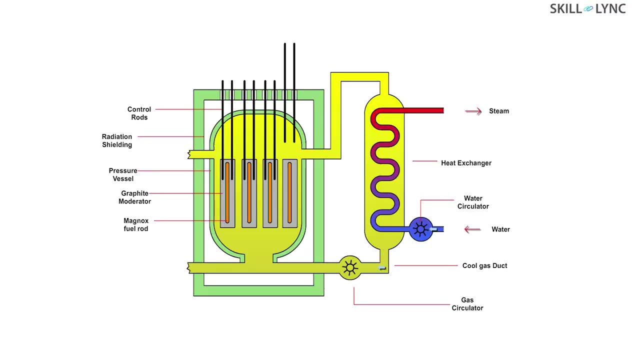 coolant in these reactors. Since the density of gases is relatively lower than liquids, sufficient neutron moderation is possible, along with better heat transfer. The fuel used in the gas cooled reactors is also different. Natural uranium is used as fuel and cladding is provided to the fuel. 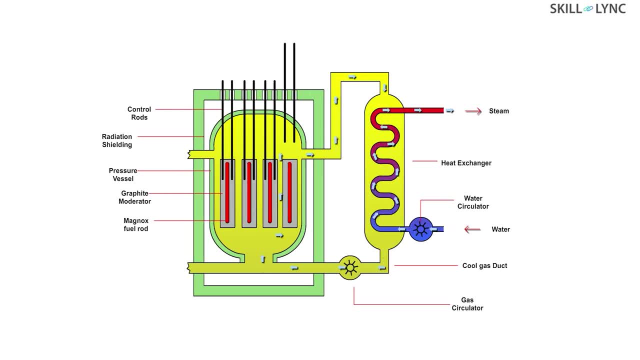 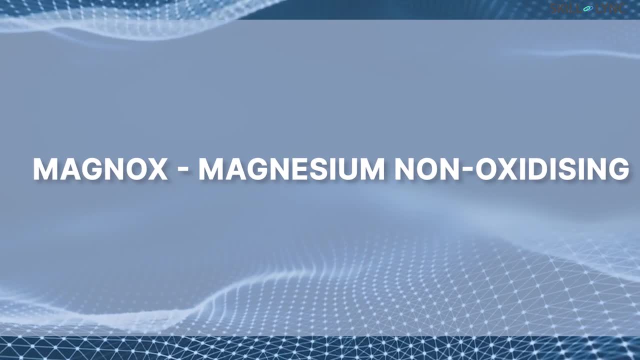 with a metal. The gas cooled reactors are also used as a coolant. The gas cooled reactors are made of magnesium alloy called Magnox, which acts as a non-oxidizing agent and reduces the reactivity with metals in the core. Hence such reactors are also called Magnox reactors In the core. 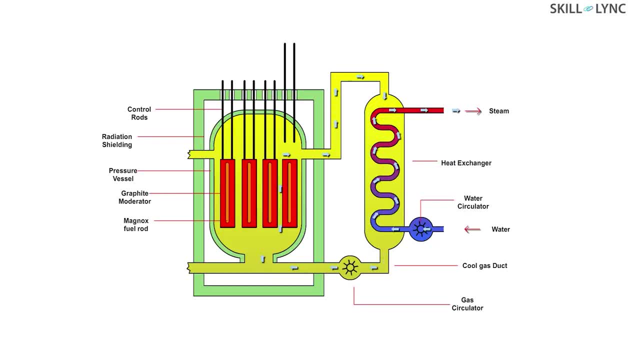 graphite is used as a moderator since it is compatible with carbon dioxide coolant. The circulator provides the coolant gas, carbon dioxide. Carbon dioxide enters the reactor core from the bottom, extracts the heat from fission and exits the reactor vessel. The gas is then. 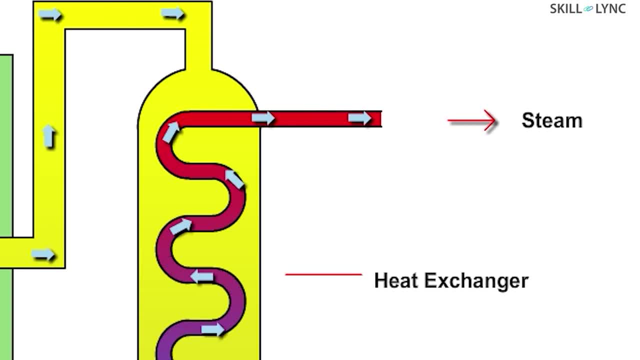 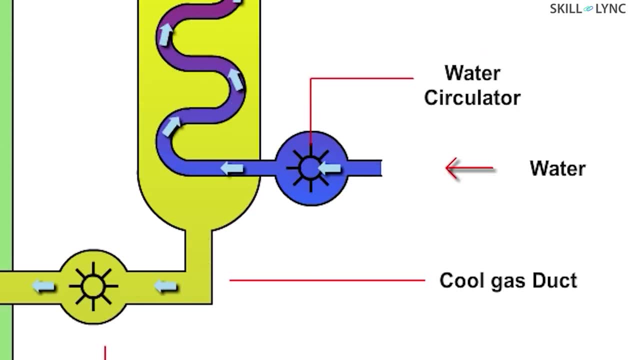 circulated through a heat exchanger that produces steam. The steam from the steam generator is then sent to the turbine for power production, and then it returns to the reactor after condensation. This is how a gas cooled reactor works, But due to the lower pressure and lower temperature of 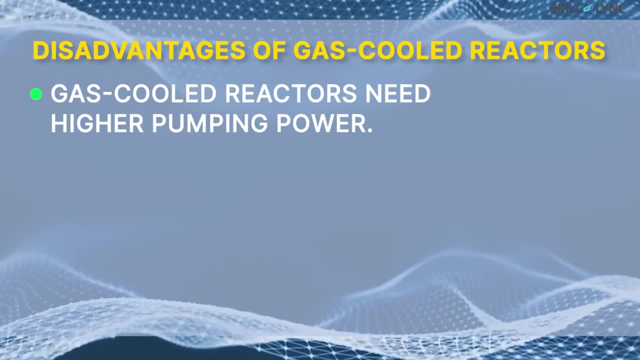 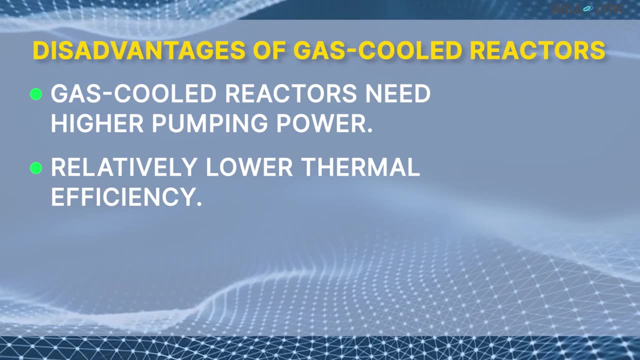 operation. such reactors need higher pumping power. Since they are first generation reactors, gas cooled reactors happen to have low thermal efficiency as compared to more advanced gas cooled reactors. To overcome this, a gas cooled reactor is used as a coolant. To overcome this, a gas cooled reactor is used as a gas cooled reactor. To overcome this, a gas cooled reactor is used as a coolant. To overcome 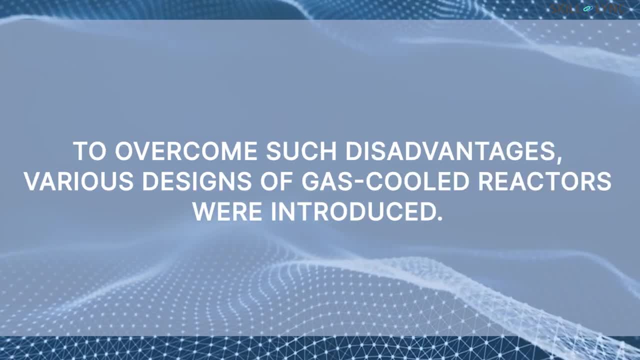 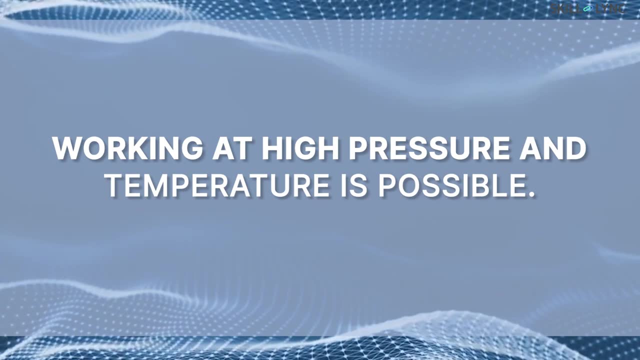 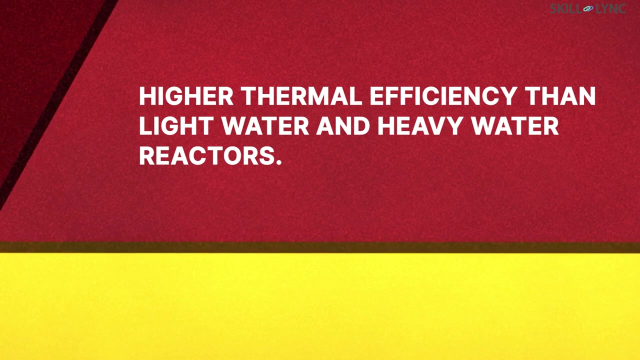 such disadvantages, various designs of gas cooled reactors were introduced. One such type of reactor, namely high temperature gas cooled reactor, can be operated at a much higher pressure and temperature by using helium gas as a coolant. High temperature gas cooled reactors also have higher thermal efficiencies as compared to light water and heavy water reactors. 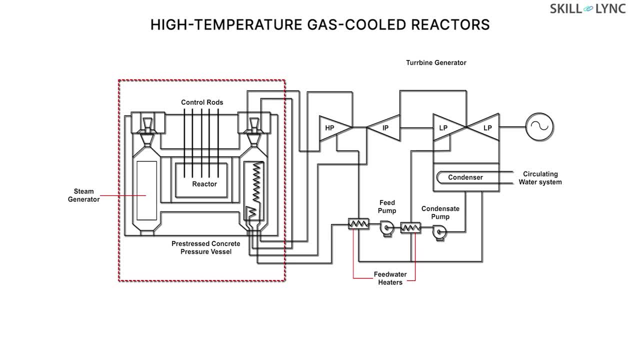 Now let's see the working of a high temperature gas cooled reactor. Similar to the gas cooled reactors, a high temperature gas cooled reactor also uses graphite as a moderator, But here helium is used as a coolant. Helium is preferred because it is an inert gas and thus 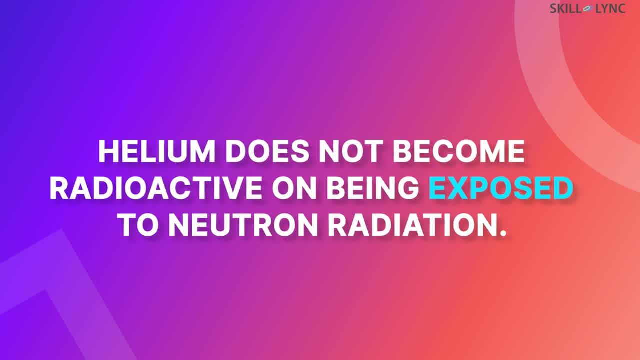 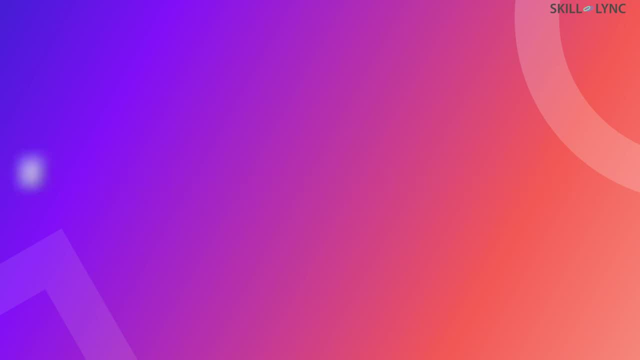 does not chemically react with the components. Also, unlike other coolants, helium does not become radioactive when exposed to neutron radiation. Moving on to the reactor core, the fuel used in high temperature gas cooled reactors is a mixture of enriched uranium, which is fissile, and thorium.